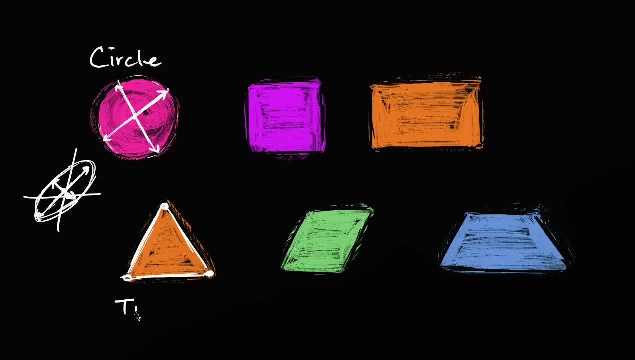 Well, if you have three sides, we call that a triangle Triangle. Whenever you see this tri right over here, that's a good sign that you're dealing with the number three. This is a triangle. It has three sides. Now, what about these shapes over here? 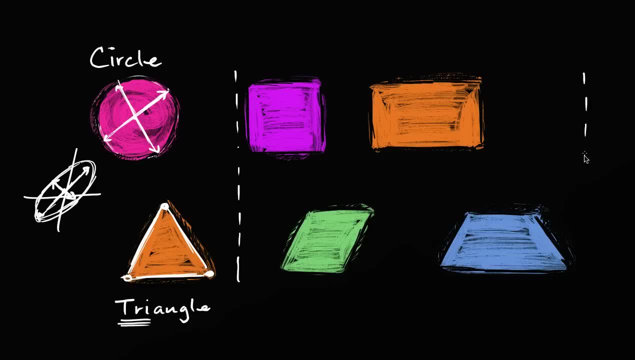 These shapes are interesting. How many shapes, sorry, how many sides do these shapes have? Well, if you count them, you see that this one up here in purple has one, two, three, four sides. This one has one, two, three, four sides. 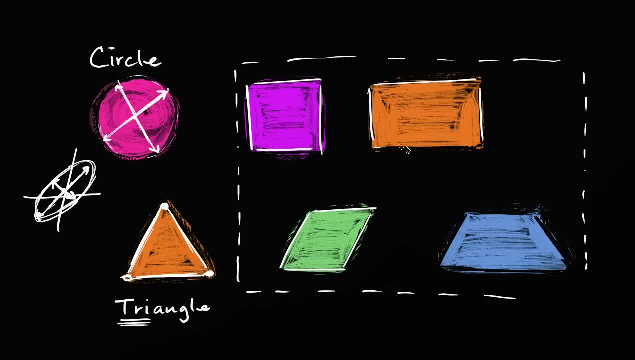 This one has one, two, three, four sides. This has one, two, three, four sides, So they all have four sides. So our name for any shape that has four sides is quadrilateral, Quadrilateral, And when you see this quad at the beginning of the word, 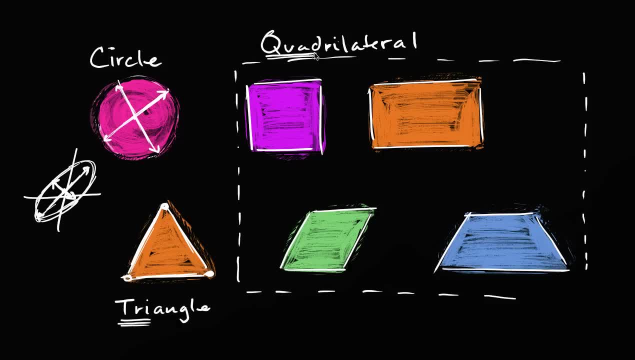 that's a pretty good sign that you're dealing with the number four. Four sides, Four sides- That's what quadrilateral means. But these are all different special cases of quadrilaterals, And actually you could even have a quadrilateral that looks like this: 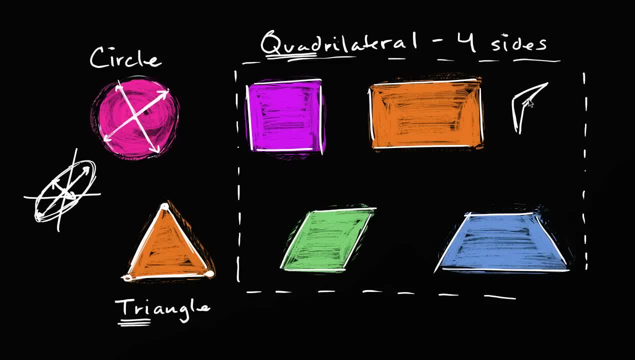 You could even have a quadrilateral that looks like this: One, two, three, four sides. As long as it has four sides, it's a quadrilateral, But let's think about each of these. So this shape right over here. 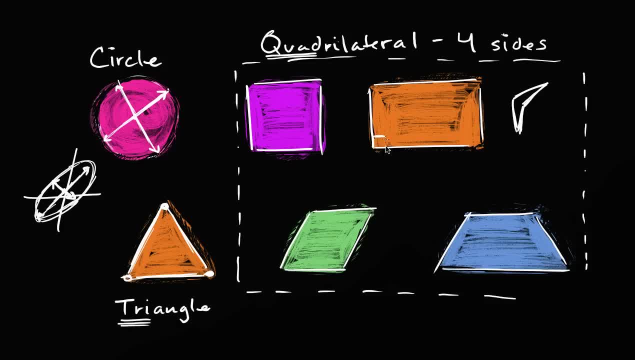 what you might see is the corners, the corners all come in. sometimes this is called square, or sometimes you could call it a right angle. So, and notice, I could put little small squares here. So if all four corners are square, 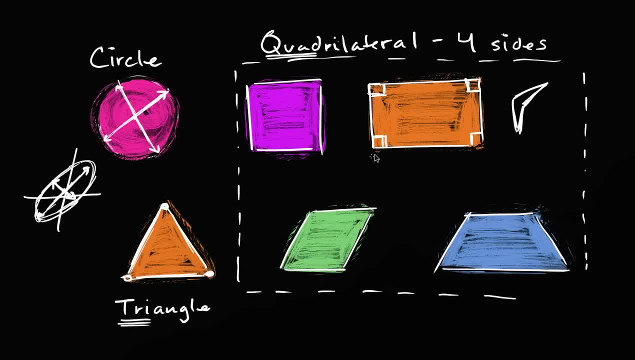 or they all come in at a right angle, like this, then you are dealing with a rectangle. You are dealing with a rectangle And so, just to be clear, this down here is not a rectangle. Notice this corner right over here, if I tried to put a little square here, 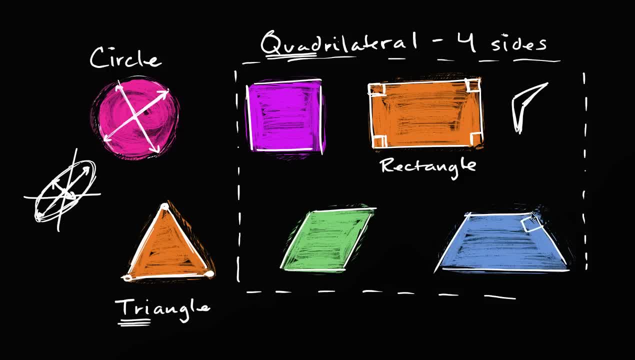 it would either look like this- and so it doesn't- the two sides aren't on two sides of the square- or it would look like, or it would look like this. So this is not a square corner, and neither is this. 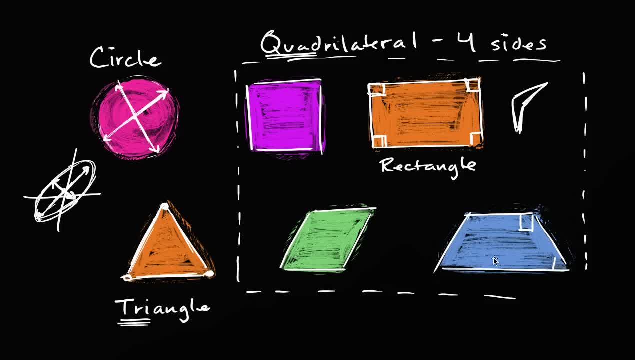 Or neither is this. So this is not a rectangle. All four corners need to be square. This one also is not a rectangle. Notice, the corners are not. the corners are not right angles. So this isn't a rectangle. this isn't a rectangle. what about this? 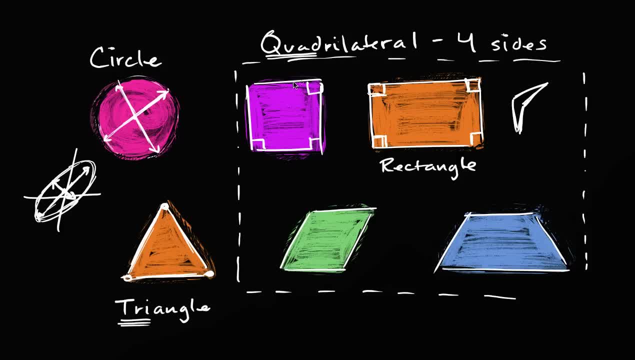 Well, I can do that. I can put little squares. I could put little squares in the corner, or I could see that they are all right. all the corners are right angles, So this actually is a rectangle as well. So these are both. 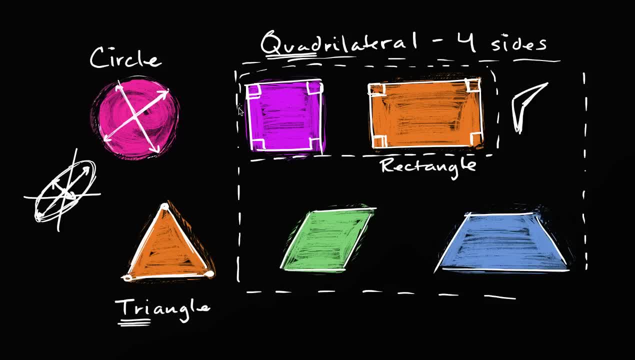 these are both rectangles. Now you might recognize this purple one on the left as a special type of rectangle. Not only are all of the corners square, not only do they have these right angles, but all the sides are the same length, or at least it looks like it from this picture. 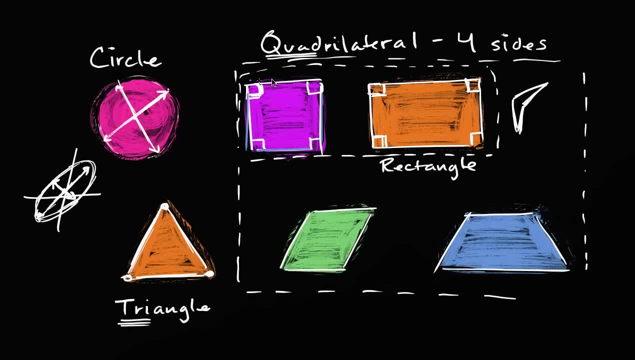 This side is the same length as this side, the same length as that side, same length as that side. So if all the sides are the same length and all the corners are square or they have right angles, well then we call it a square. 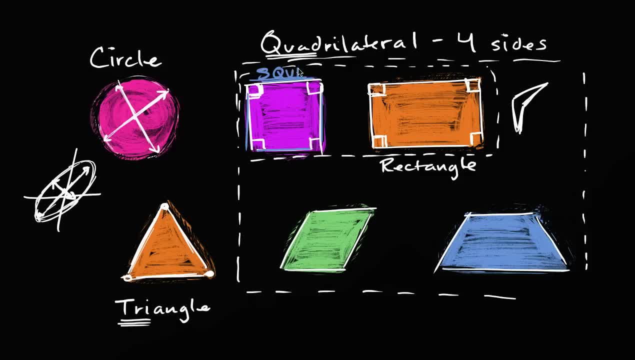 So this right over here is a, this right over here is a square, special type of rectangle. This one: not all the sides are the same. this one, all the sides are the same. Now, what if we go down here? It looks like all the sides are the same. 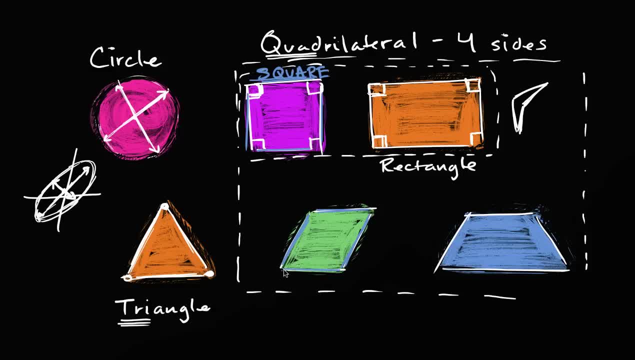 one, two, three, four, but it doesn't have square corners. Notice, if I try to put a little square here, it wouldn't fit perfectly. If I try to put a little square here, it doesn't fit perfectly. These aren't right angles. 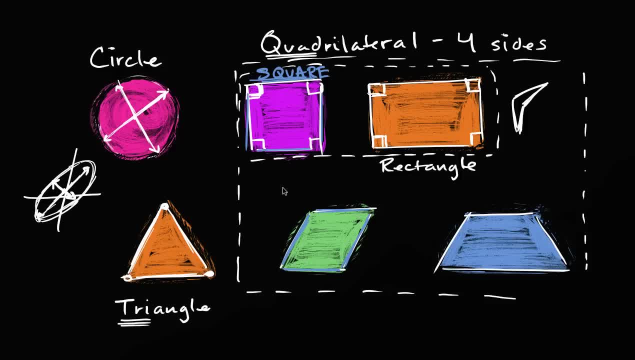 So if all four sides are the same, and that's all we know about it, we call it a rhombus. We call it a rhombus. So you might be saying, wait a minute, this square, all four sides are the same. 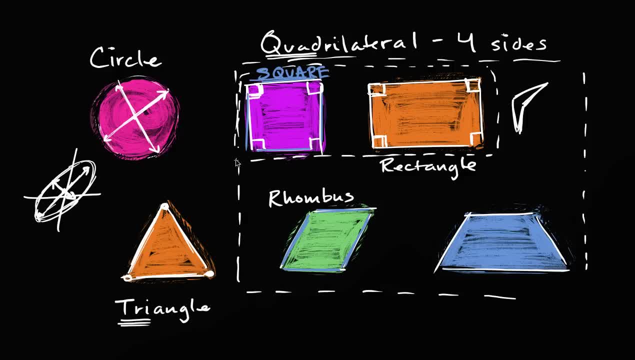 is that a rhombus? Yes, it is. So the square is a rectangle, it's a rectangle and it is a rhombus. So this last shape here, this last quadrilateral. what's interesting about it is you have two of its sides. 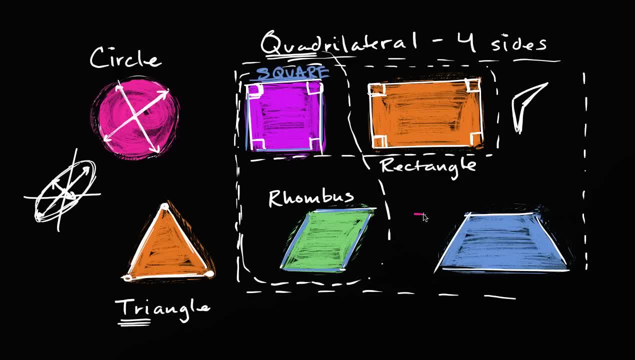 going in the same direction, So this one right over here. notice what I mean by the same direction, and sometimes this is called parallel. If I draw two lines here, these two lines are never going to cross each other, So these two lines are parallel.